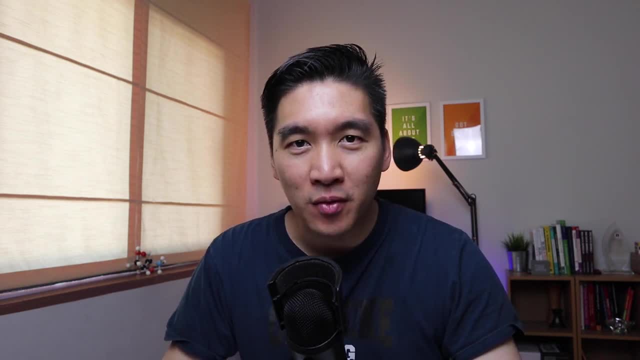 Welcome back to the Data Professor YouTube channel If you're new here. my name is Chen-Ninh Nantat Senamat and I'm an associate professor of bioinformatics. On this YouTube channel we cover about data science concepts and practical tutorials. So if you're into this kind of content, 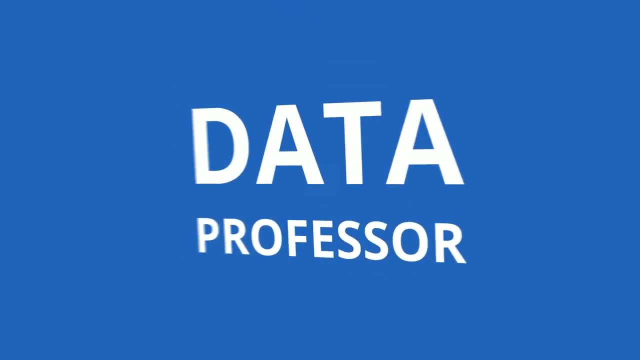 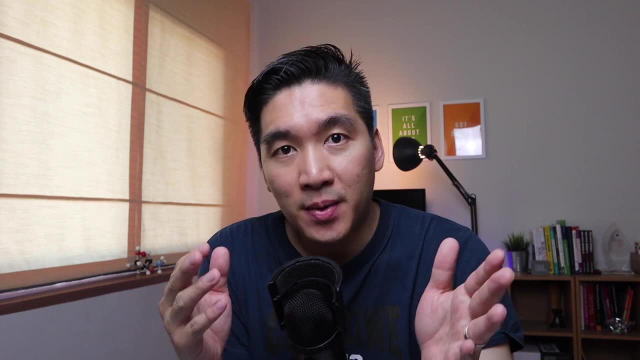 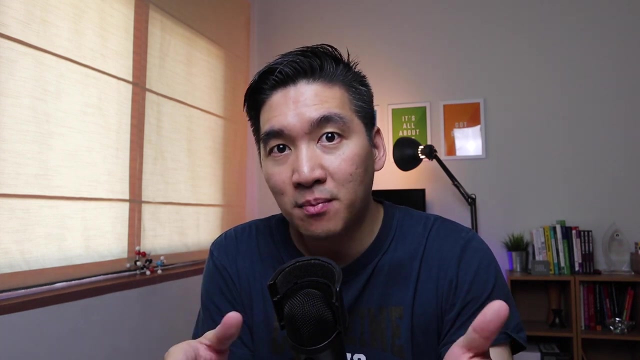 please consider subscribing. So I have been mentioning for quite some time about making Python tutorial videos, And so today is going to be the first episode, and we're going to look at how you can build a simple classification model using random forest algorithm on the Iris dataset. 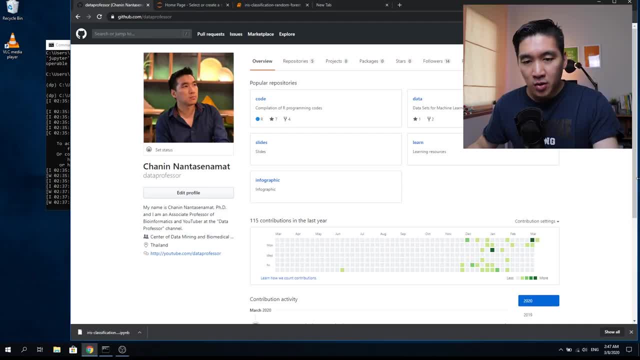 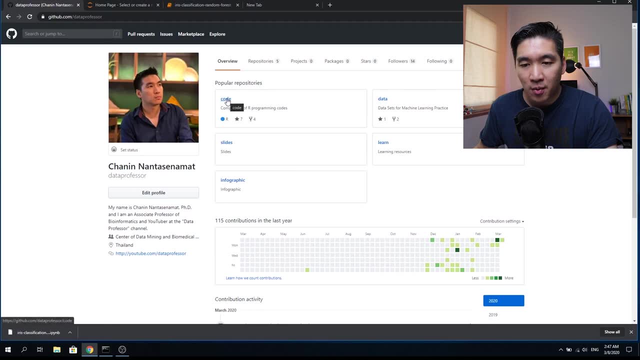 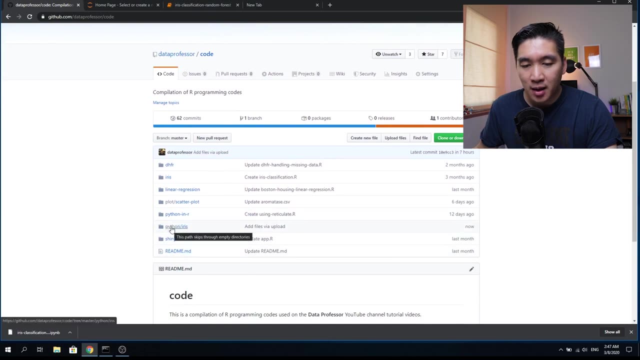 So, without further ado, let's get started. So why don't you go ahead and open up the GitHub page of the Data Professor and click on the code repositories, Scroll down and then find the Python tutorial, Iris? So, because the Python repository contains only one subdirectory, it will show it as a Python. 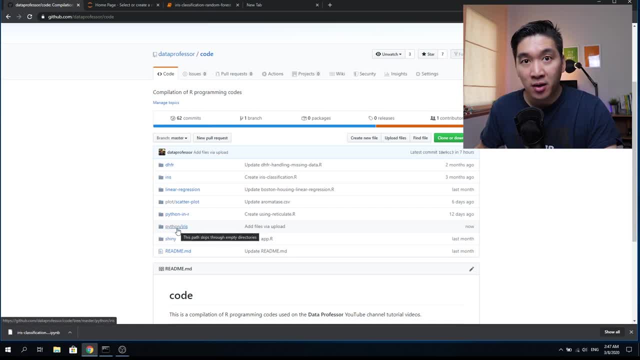 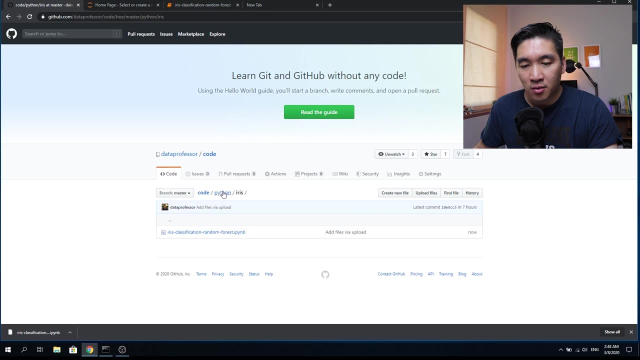 slash Iris, But in the future, when there is more video in the Python subdirectory, the name Iris will disappear and it will only appear as Python, So you can just click on it. Okay, and then you are inside the Iris subfolder of the Python repository under the code repository. 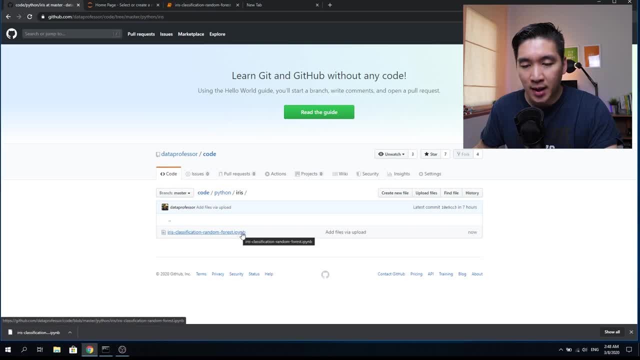 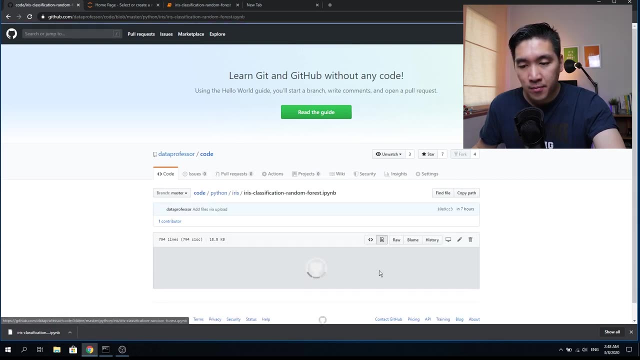 So in here there is one file called the ipynb. So the ipynb is the file extension for the IPython Notebook, which is the original name before it became Jupyter Notebook, And so what you want to do is click on this file. So the advantage of having Python codes in the Jupyter notebook is that the 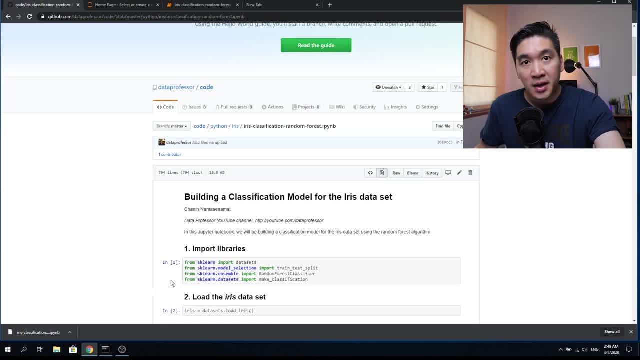 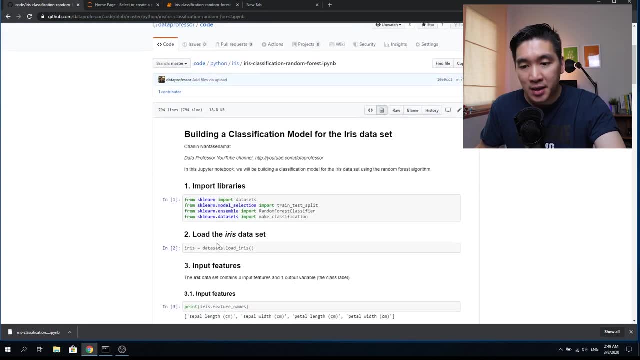 input code and the output code can be shown on the same page without any compilation or running the code on a local computer, And so therefore, my notes there in here will stop working. So now to a local computer, so you can even look at this on your tablet, on your mobile phone. 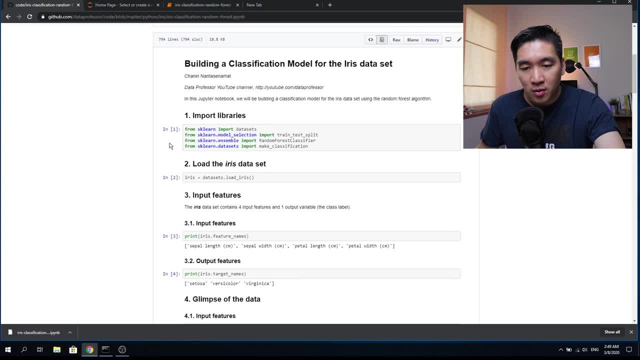 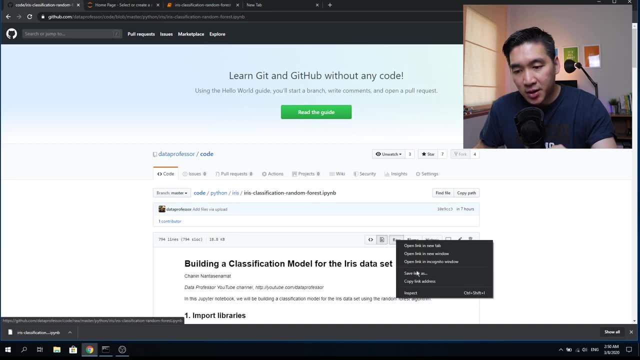 when you're on the go, so you will comprehend what input will lead to what outputs. okay, so what you want to do now is right click on the raw link and then save link as or save target as: okay, find a suitable location on your computer and then save it in there. so I have already saved that, so I will just open up the. 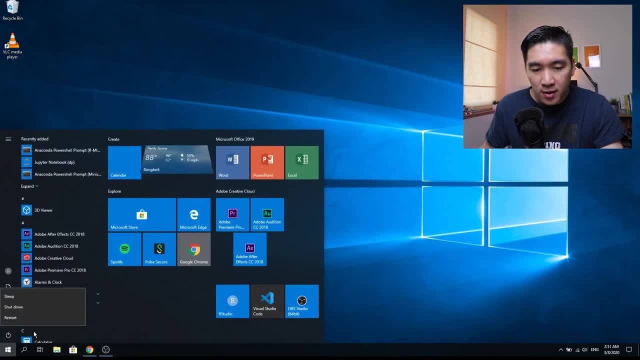 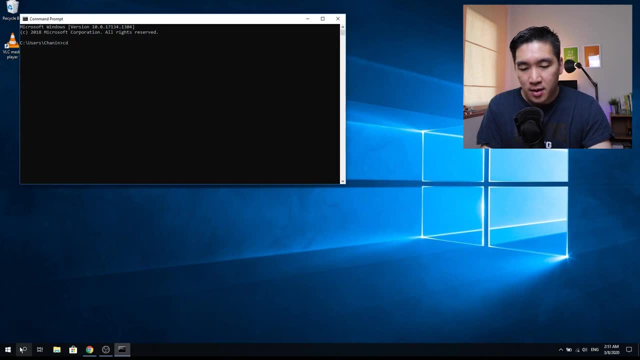 file. then I'm going to fire up the command prompt and then I'm going to go into the directory where the files are located and then I'm going to activate my conda environment and then I'm going to run the Jupiter notebook, okay, and then I will see the. 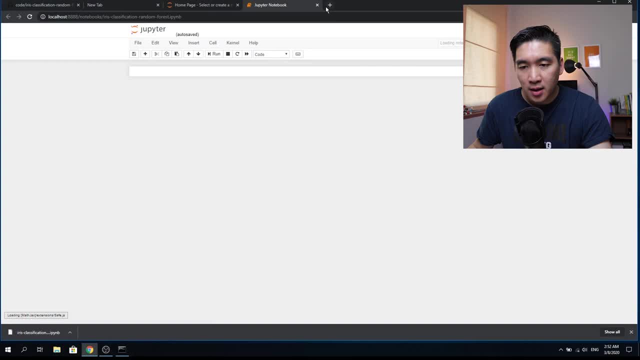 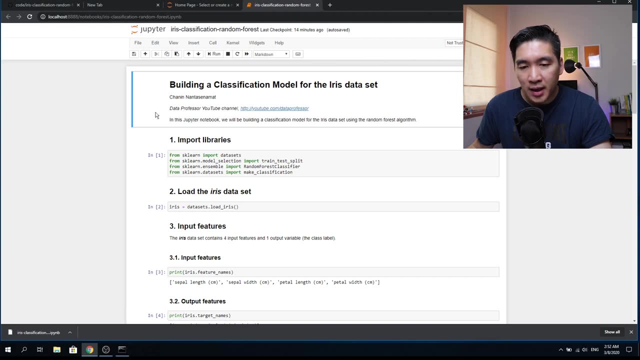 Python notebook file here. click on it and then it will load up. okay, so you can see that this Jupiter notebook looks like a document, so it is a blend of Python code along with documentation, and the documentation, as you see here, could be written in markdown language or using HTML. 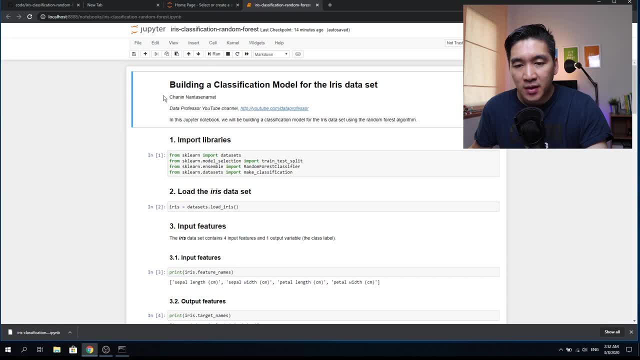 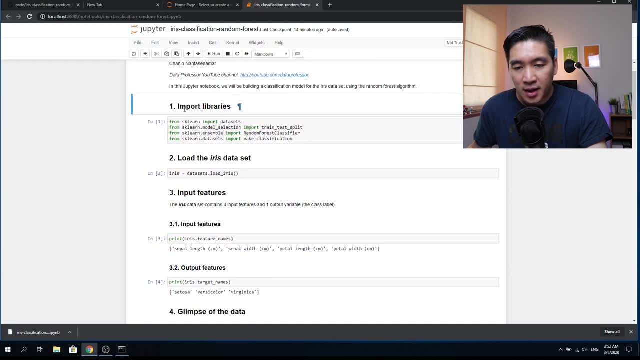 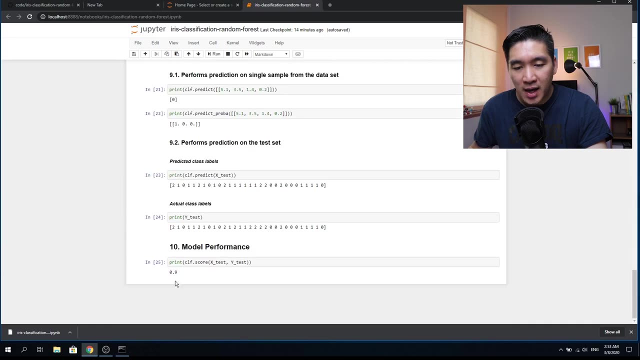 So the first cell provides the title of this Jupyter notebook file, And then the second cell we see here is the header, and then I number it for easy reading. So the first section here is called import libraries, And we will see that there are a total of 10 steps that you could do. 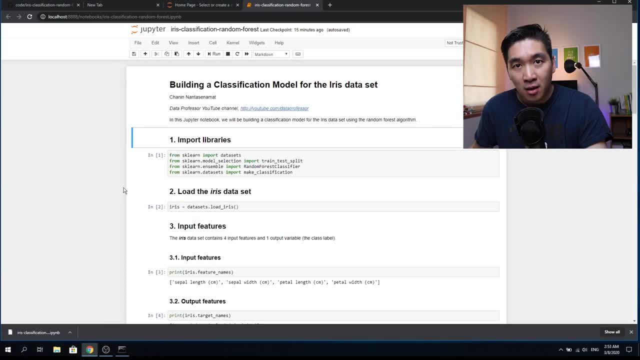 to build your first classification model in Python using random forest algorithm on the iris data set. So the first step is pretty easy. you're going to import the libraries, and the libraries that we're going to use today is based solely on the scikit learn package And scikit. 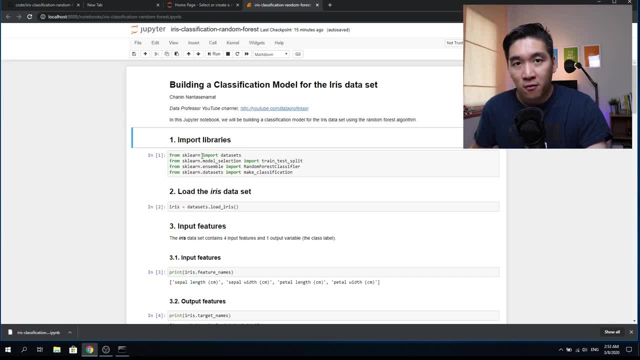 learn package is a popular machine learning algorithm package for the Python environment. So we're going to use scikit learn to import the data set iris, which will be taken directly from the data set sub module of the scikit learn, And then we're going to use the train test split function. 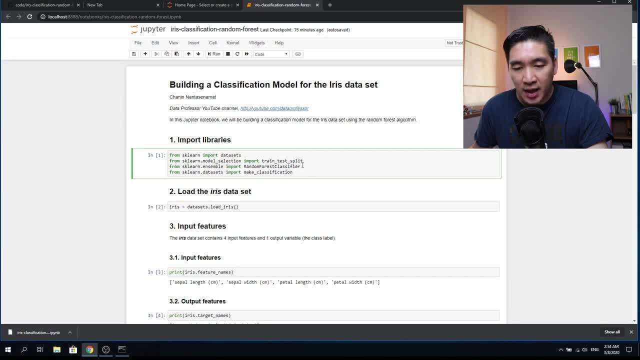 and as well as the random forest classifier and the main classification. Okay, and then the second step is to import the data set iris, And then we're going to import the data set iris. And then the third step is to load the iris data set, And we're going to do that by assigning the iris. 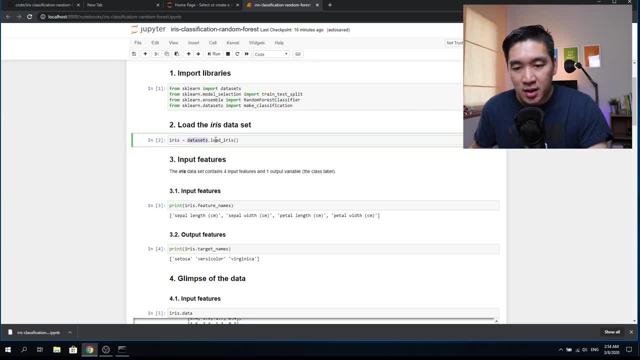 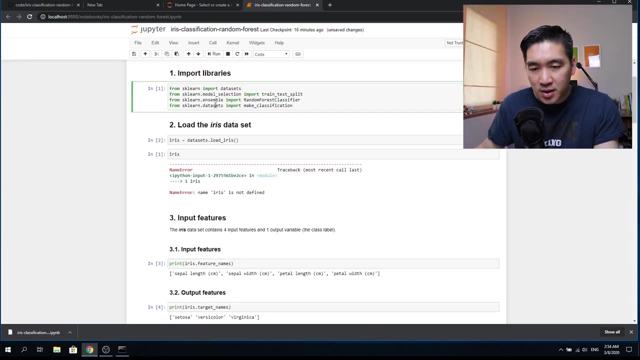 variable with the data sets function and then load iris function. we're actually it is the data set sub module And within it we're going to use the load iris function. So this will put the iris data set into this iris variable. So in order to run the cell, you want to click on the cell And on. 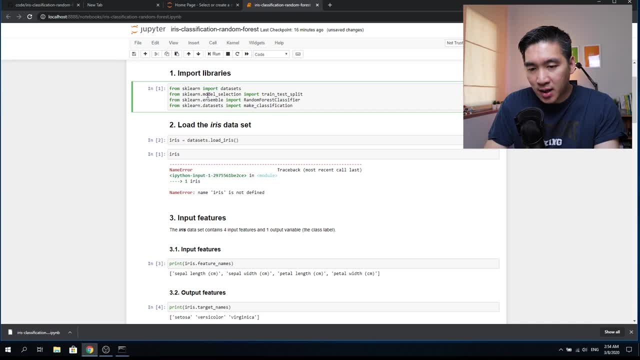 the keyboard, press and hold the Shift key along with the Enter key, And then you will see that, briefly, the number will appear to be an asterisk, which means that it is currently running, And when it is completed it will become a number. the number will be done sequentially, So 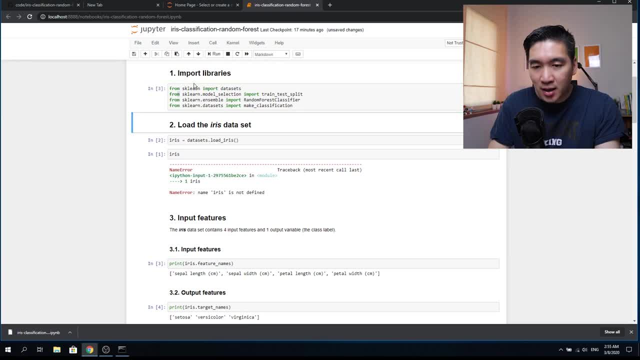 this is the second time the cell has been run, So if I run it again, it will become three. Okay, so now we're going to load the iris data set And you see that the number become four, which continues from the previous cell, which is three. And so let's enter iris And let's 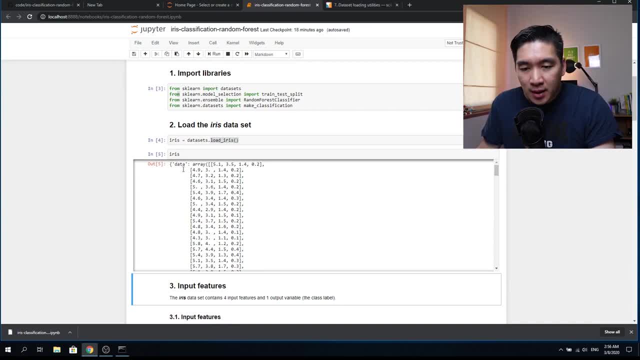 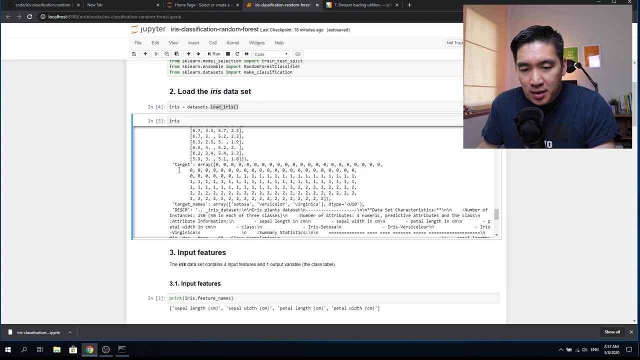 see what happens, Okay, and then we will see that underneath there is the data set iris. And then we will see that underneath there is the data set iris. And then we will see that underneath there is the data, Which comprises of 150 flowers, the target, which is the class labels, and. 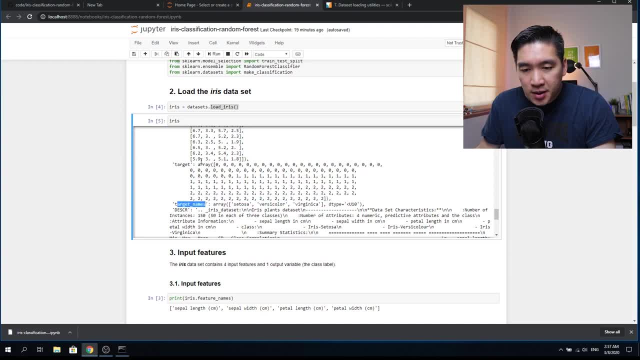 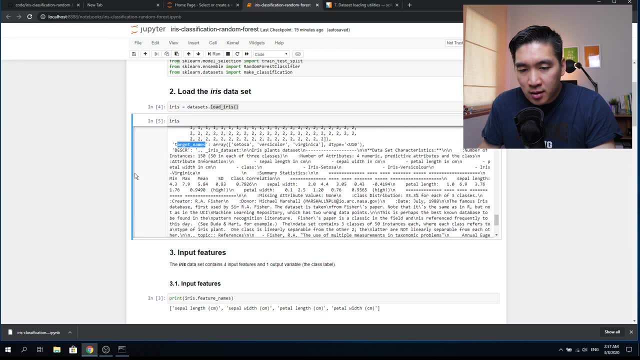 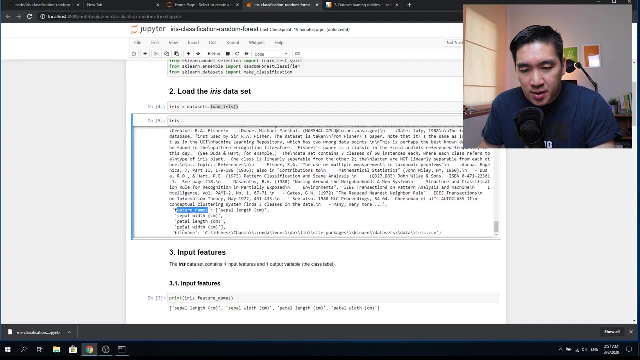 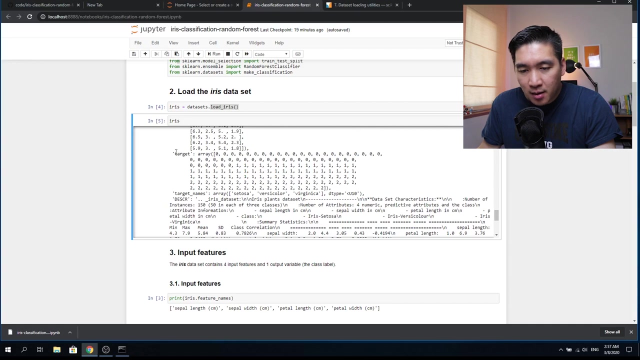 the target names, So 012 corresponds to COSA, versicolor and virginica. And then this is the description of the data set And then the feature names, which are the steeple with pedaling, pedaling width and also the simple length. So what we can do is we could call it by specifying iris dot. 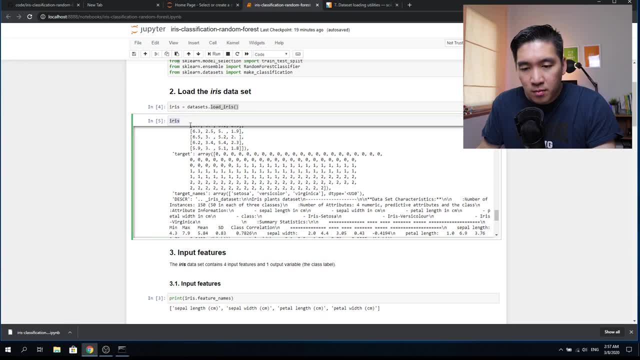 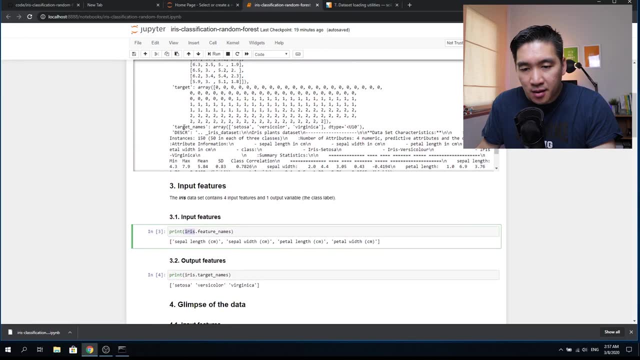 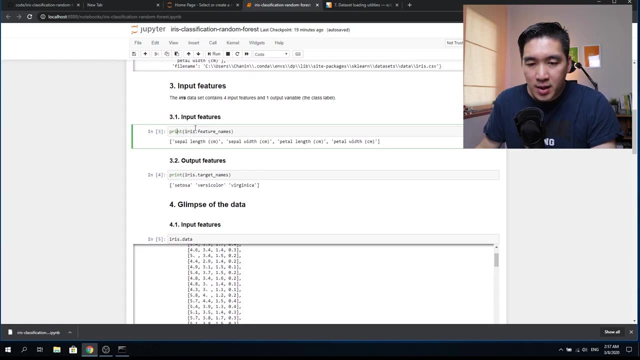 target, which we will do below. Okay, So let's go ahead and specify that, as we see that there is a feature name here. So we're gonna print iris dot feature names which will allow us to see the input features which will comprise of the four characteristics of the iris flower, which are: 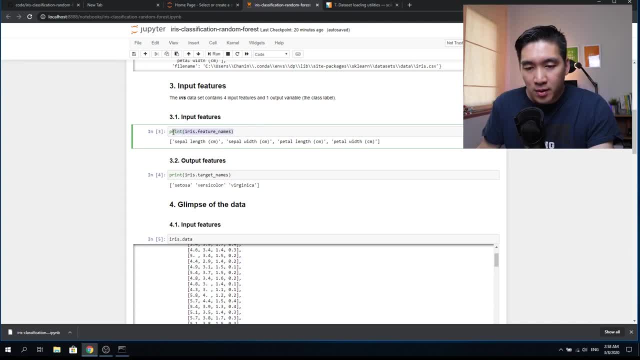 the simple length, simple width, petal length, petal width. So when we shift, enter, we're gonna get the same result as it was done previously. And then to see the output feature, it is in the iris dot target names And actually if you want to add a cell we can click on the plus button here. 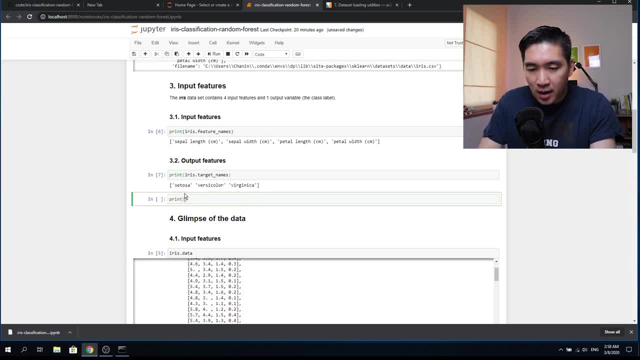 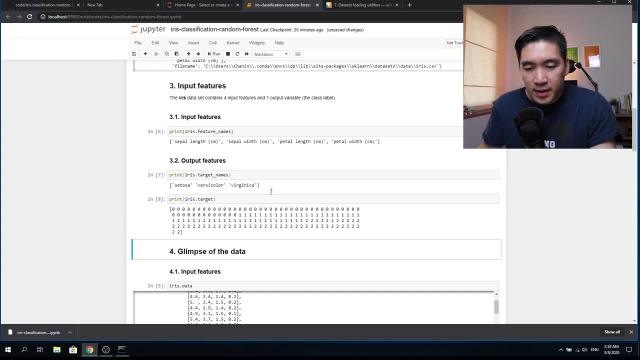 And it will add a cell So we could type in iris, dot, target, shift, enter, and then we're going to see the 012.. So it's going to be the same thing, But this will be numerical or integer, But this will. 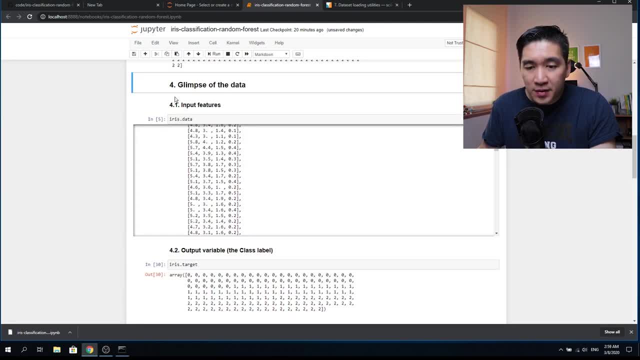 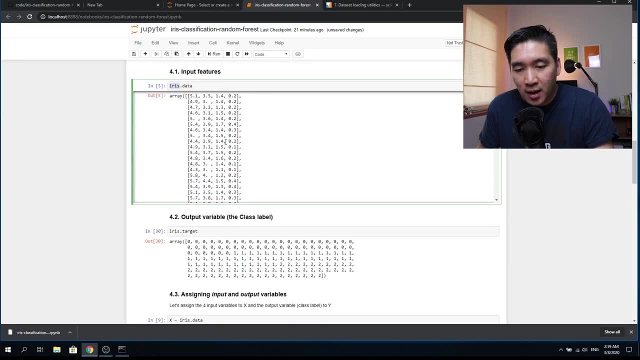 be the strings version. Okay, in the fourth step we're going to take a glimpse at the data, So iris dot data, and then we're going to see the data here as an array And then, okay, so this we have done previously above. Okay, so go ahead and assign. 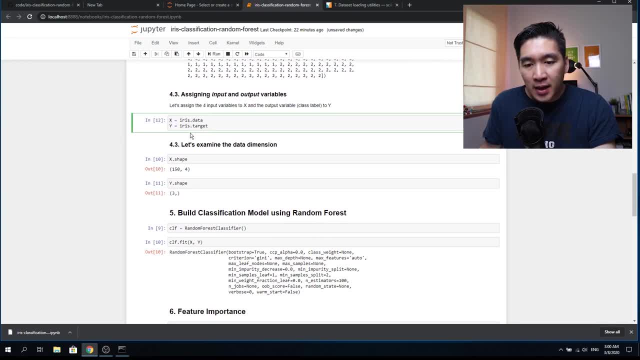 the iris dot data into the x variable and assign the iris dot target, which is the class label, into the y variable. So the x will contain four input features and the y will contain one feature. So it will add up to a total of five features and 150 data samples representing 150 iris flowers. 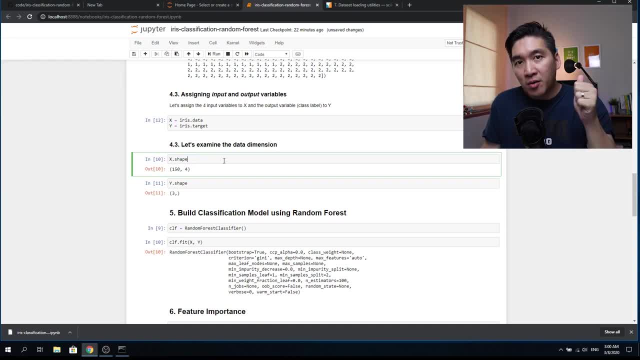 where it belongs to either one of three classes: iris citosa, iris versicolor and iris virginica. So if we look at the data dimension, we will see that there are 150 roles and four columns, So corresponding to 150 flowers. 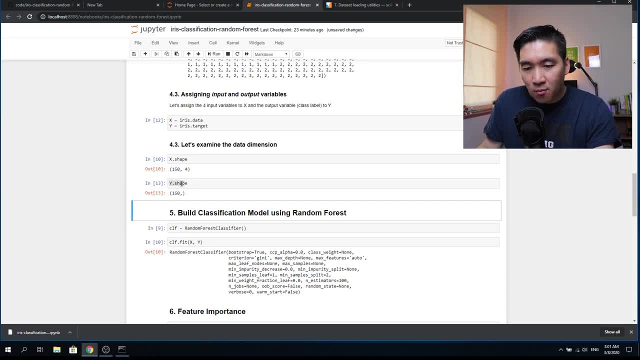 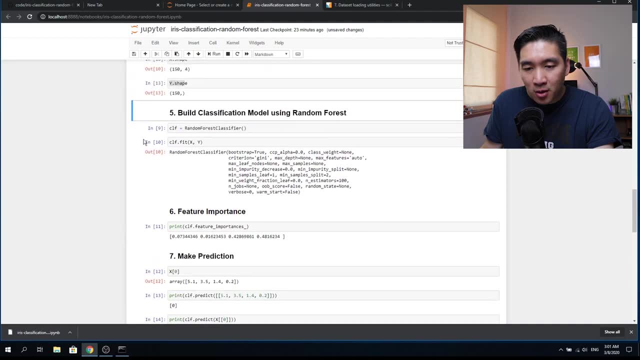 and four input features, and then the y shape will become 150.. So nothing is shown afterward because it is one column. Okay, now comes the fun part. we're going to define CLF, which would stand for the abbreviated form of classifier, And we're going to use the random. 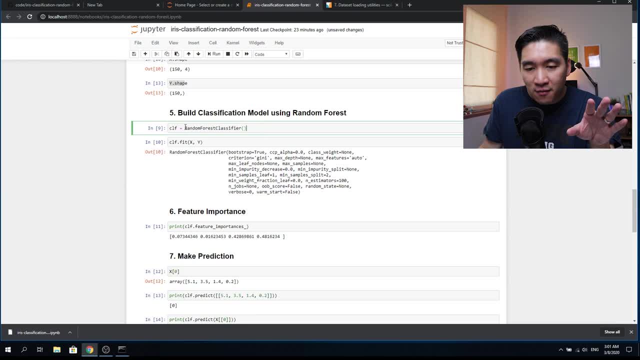 forest classifier function. And then we're going to call the random forest classifier function by typing in CLF and then dot fit, And then as input argument we're going to use x and y. So what this essentially does is it's going to call the classifier, which is the random forest classifier. 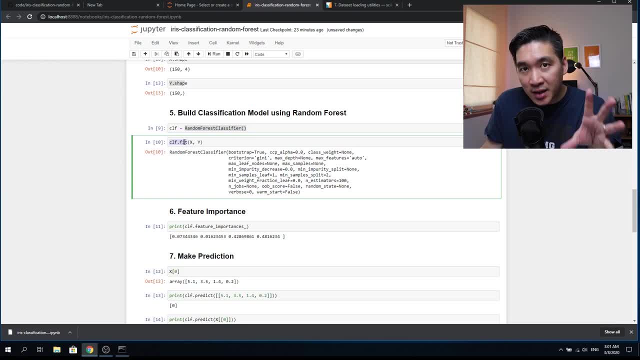 And then it's going to use the fit function, which will create a classification model, And then it will take as input two variables. The first one is the x variable, which are the input features, And the second argument will be the y variable, which is the class label. So it's going to take in x and y. 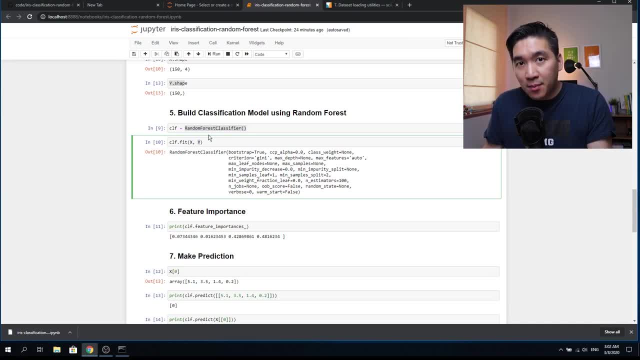 Create a model by using y as the class label. So the model will be performed in a supervised manner by learning from the class label and finally outputting a classification model using the random forest algorithm. So we're going to see that under the hood, it's going to use these. 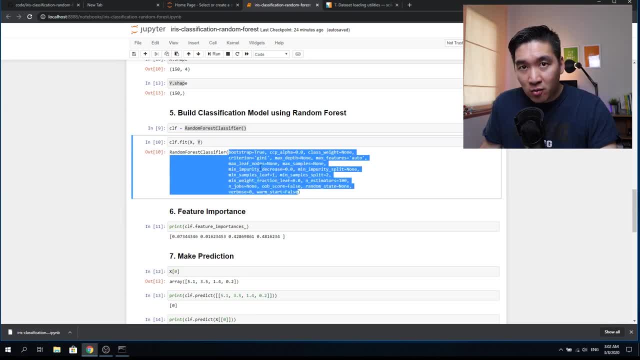 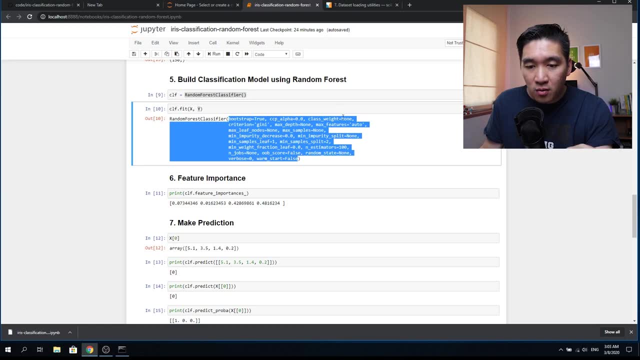 default values which you can modify later on to your own personal liking. So we're going to cover in more depth on random forest algorithm later on, in a future video. So let's go ahead and look at the feature importance. So these are the important features. So let's have a look. 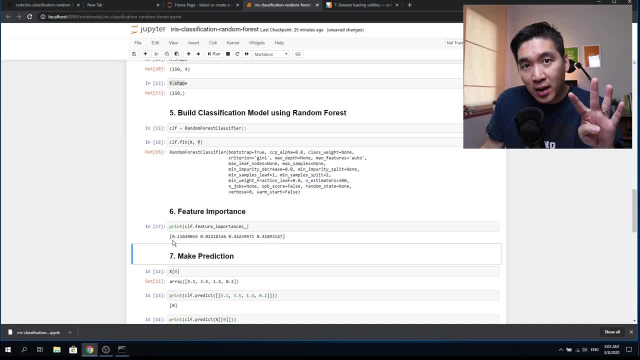 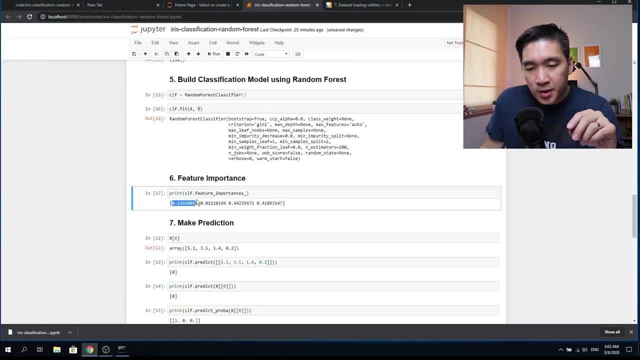 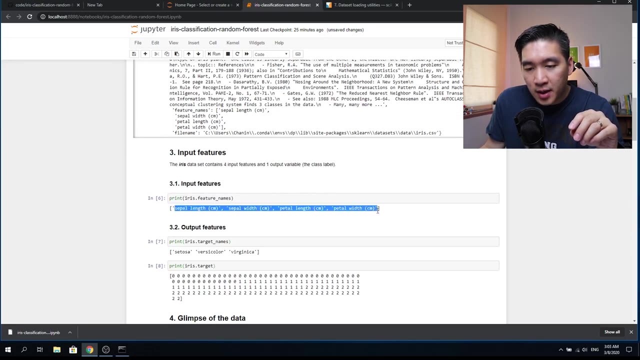 So we have four input features- the simple length, width, the petal length, width- and each of them have corresponding importance to a different degree to the classification model. So the values are in order for the respective input features that we have here. Okay, so the importance of each of these variables will: 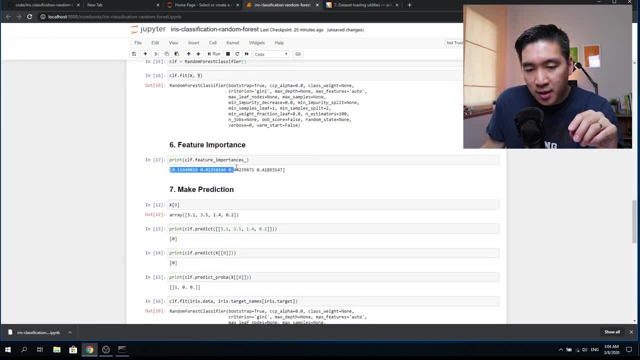 be in order for the respective input features that we have here be shown by the number, And it's right here. So we can see that the most important feature was the third variable and then followed by the fourth variable and then the first variable. 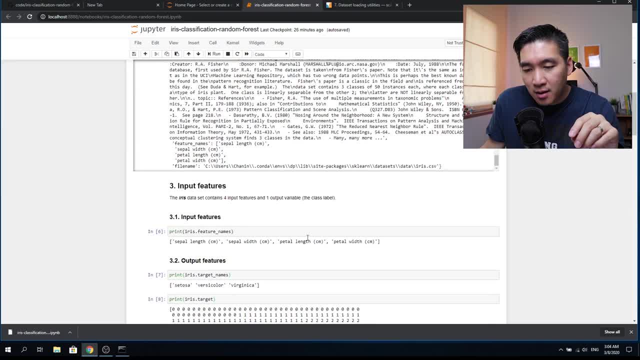 So the third variable is: the petal length is the most important, as suggested by the model, followed by the petal width, followed by the simple length And the last important feature is steeper width, which is, but it contributes to a lesser degree to the classification model. 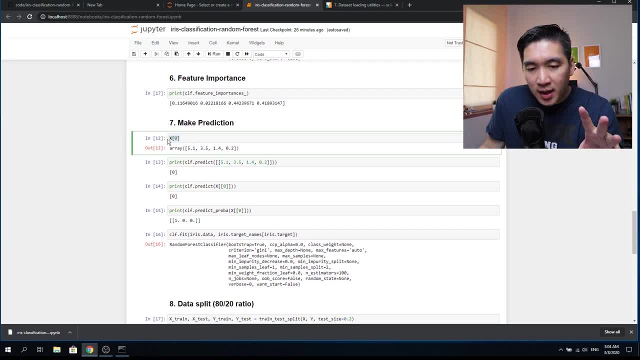 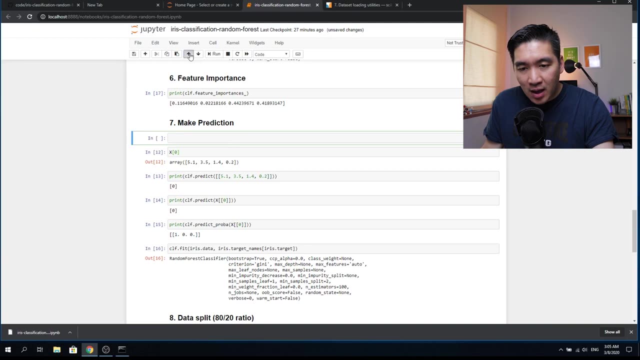 And so. so let's make a prediction And we're going to feed in the first data sample, which is the first flower. as we recall, there are 150 flowers and the input data is assigned to the x variable. Let's have a look So you can see that we can move up and down the cells. So let's have 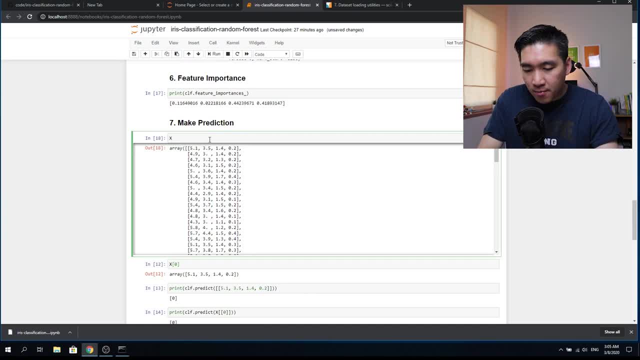 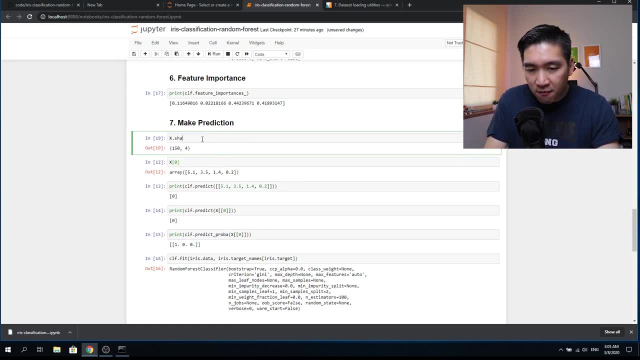 a look, x are the input features, And there are 150 flowers, And so here we're going to use the first flower, So we can just call it by using the bracket, and then zero is the first position, and we're going to get that right. if you change it to the second position, you will get a different. 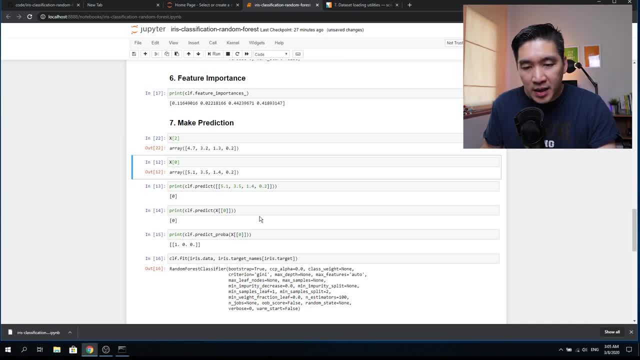 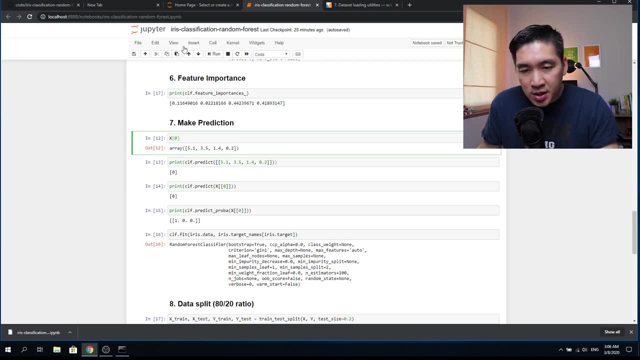 set of values. So Python counts from zero as the first iteration and we can cut it out. we're going to print the results using the print function. So the print function is just essentially printing out whatever we put in as the arguments. So if we say five, it'll print out five. 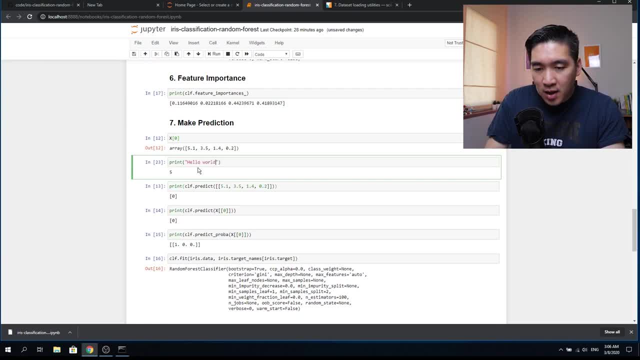 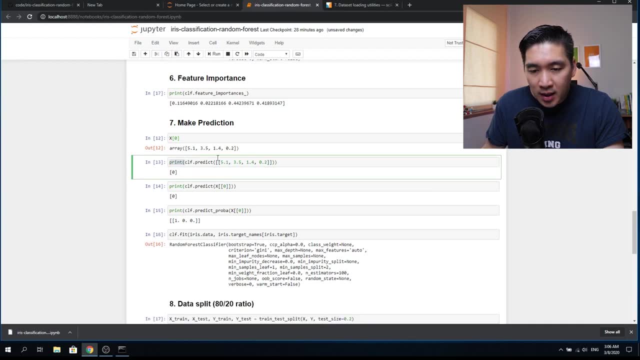 if we put in a string, it'll output a string. hello world, okay. And so here we're going to print and then taking in as argument, the prediction function of the classifier, And as input of this, we're going to put in the the set of values for the first flower. 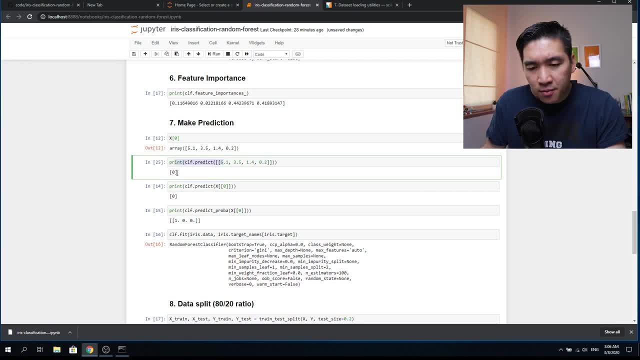 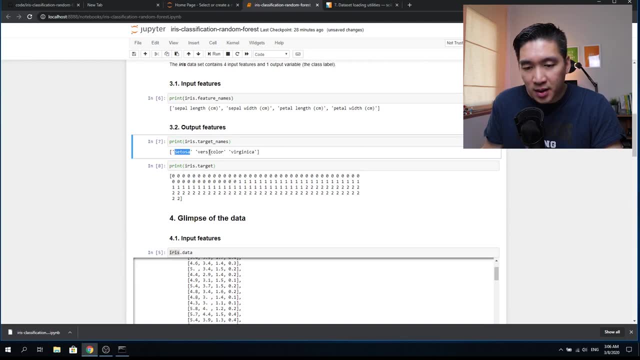 and we're going to see the prediction coming out And it prints out zero, and zero means the first class, right here, zero. So it is the setosa, right. If it's one, it becomes the versicolor, right. If it's one, it becomes the versicolor. 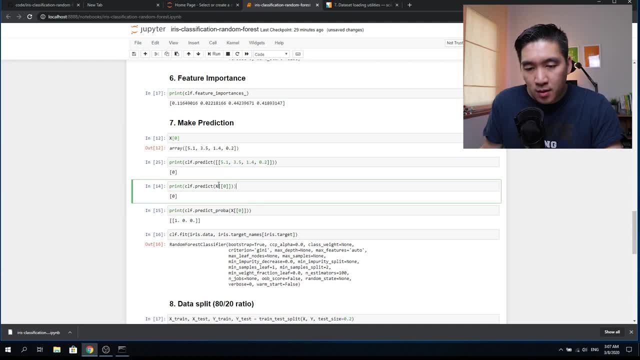 And then, with the version I got, okay and we're going to use this, which is essentially the same thing. we could put in the set of values directly, or we could just slice it directly from the x variable. So this will also give us a prediction of zero. And what about if we want to look at the 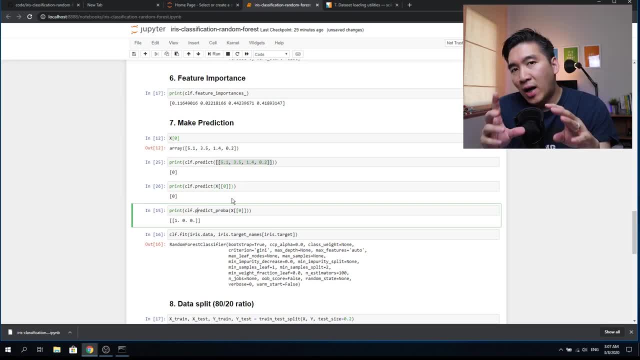 probability of the prediction we want to see before it derives at its conclusion that it will predict it to be the first class label. And let's say that it predicts the data sample to be class 1. let's say 84.. let's say 80% And the probability of being class two, 20%. Is that the case for this one? So let's. 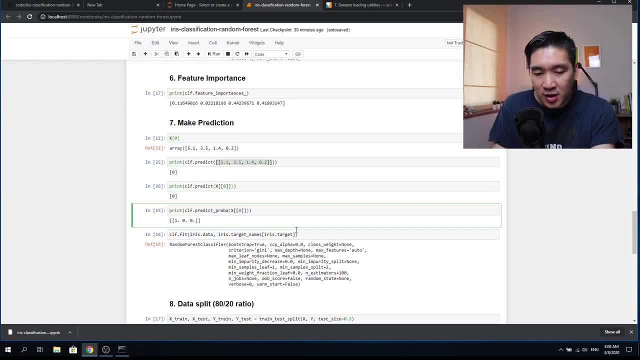 check it out And then when we run it using the predict proper function, we see that the probability to each of the three classes are shown below 100 means that 100% of the probability goes to predicting the first class. Okay, so it is 100% confident that class one, or DC Tulsa, is the. 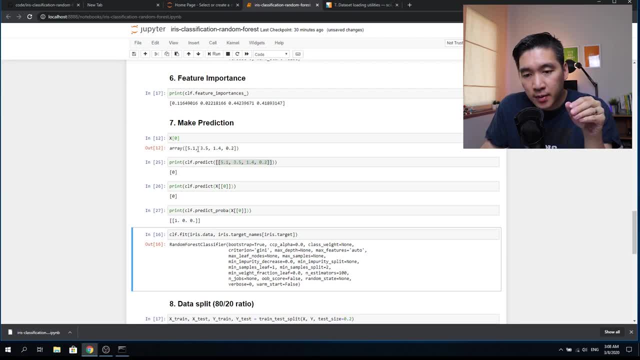 correct class for this input feature shown here in the first flower. So it is confident that the first flower with the set of values shown here is corresponding to the first class label, which is the set Tulsa. So, based on the input values of simple length, with petal length with 5.1, 2.5, 1.4. 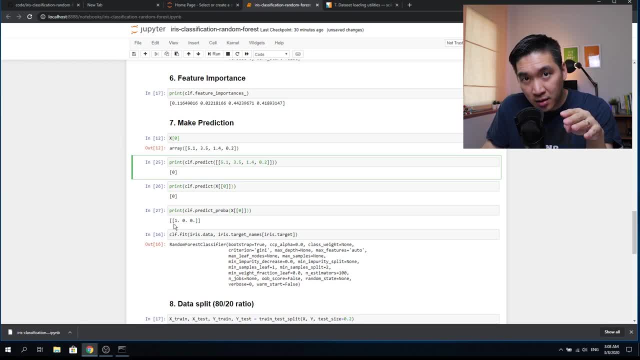 3.2, it predicts it to be iris set Tulsa. Okay, but it's a bit difficult to look at the class label by seeing just 012.. So why don't we run it using the predict proper function? So let's run this function And then we're going to see the names of the class label. Okay, there you go. 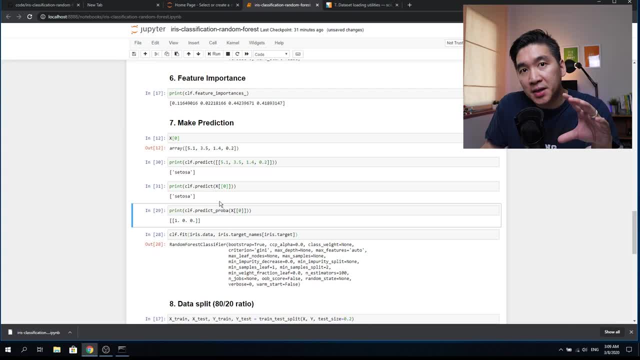 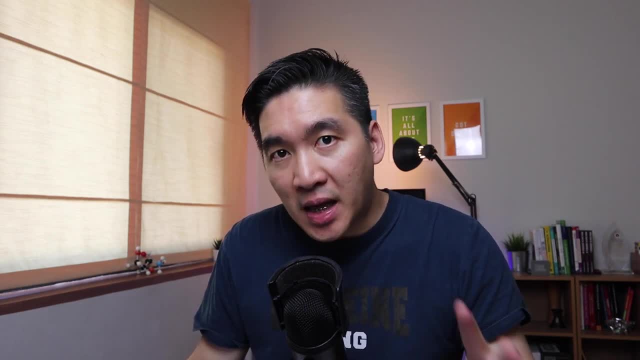 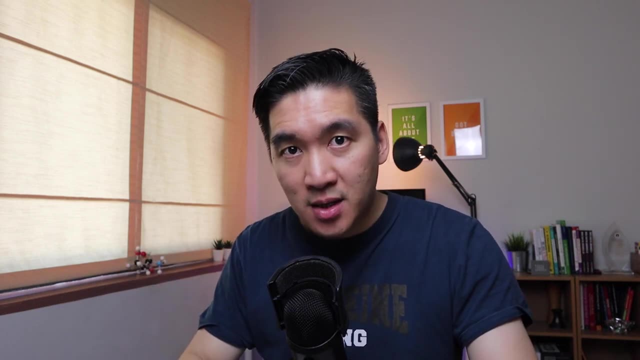 So instead of zero, we're going to see the actual class label name by using this function here. Okay, so in the previous example we use the full data set to build the classification model. But let's say that we want to use a subset of the data set. let's say we want to do a 8020 split where 80%. 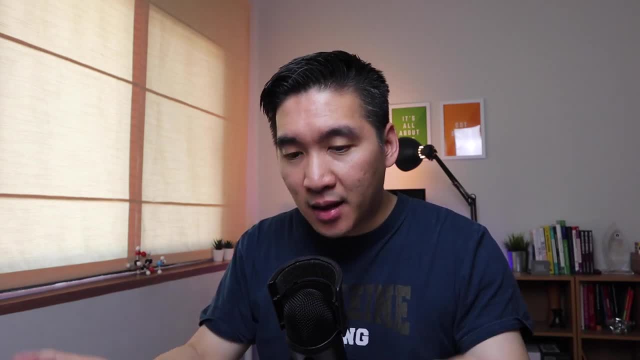 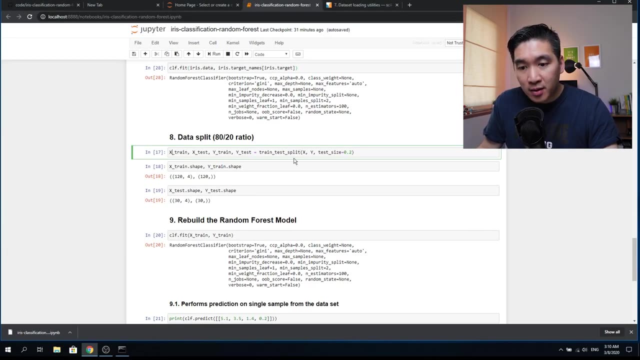 will go to the training set and 20% will go to the testing set. So how do we exactly split the data? So we're going to use the train test split function in the psychic learn and we're going to assign it to four variables, And so they're going to be called x train, x test, y train. 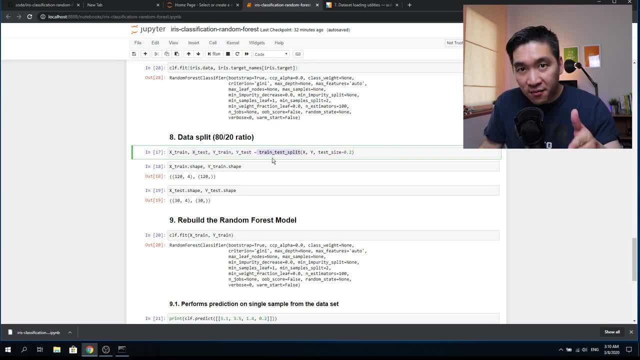 and y test. So it will take the data directly from this function, where it will specify the input argument as follows: which will take the x variable, the y variable and then the input argument of the test ratio of the train and test set Splitting ratio of 0.2, meaning that 0.2 will be for the test and 0.8 will be for the train. 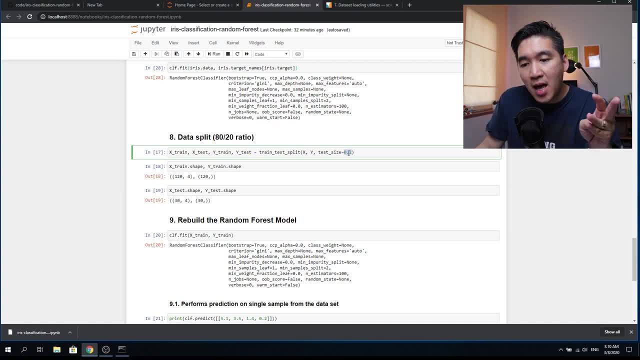 And so training set, we'll get 80% of the data samples, and 20% of the data samples will go to the test set. Okay, so let's run that. So let's have a look at the x train and y train dot shape. 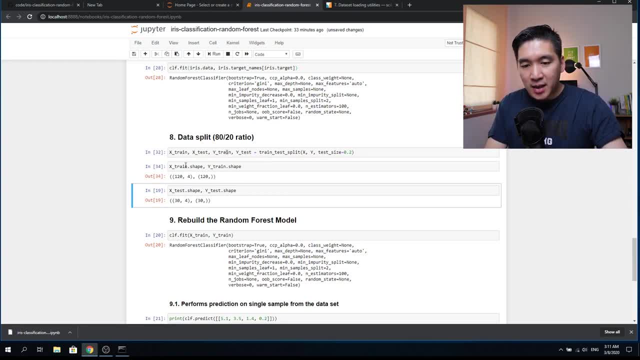 So we're going to see the dimension of the variables And we see that there are 120.. flowers and four features: for the x train And for the y train there is 120 flowers and there is one column or the class label. So that line is about the training set And then 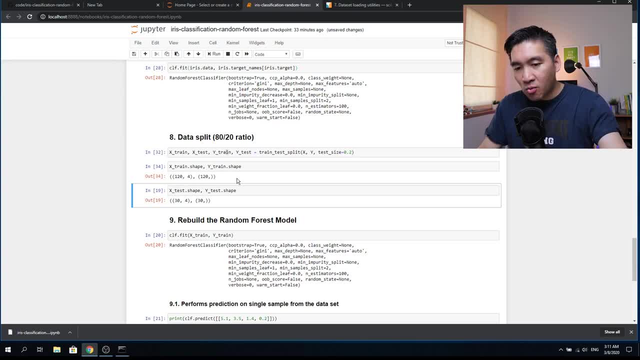 the testing set is what follows now. So x test and y test dot shape will give us 30 rows and four columns, corresponding to 30 flowers and four input feature. And then the second one for the y test dot shape will be 30 flowers and one column, which is the class label. 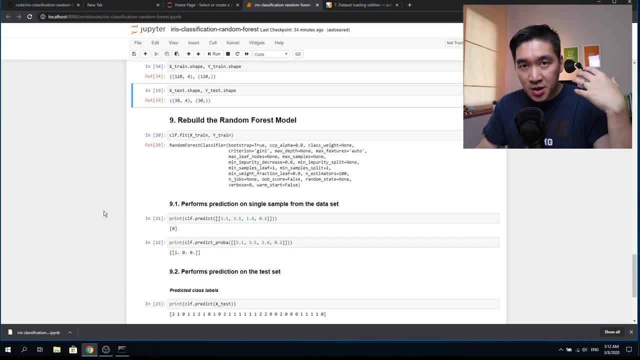 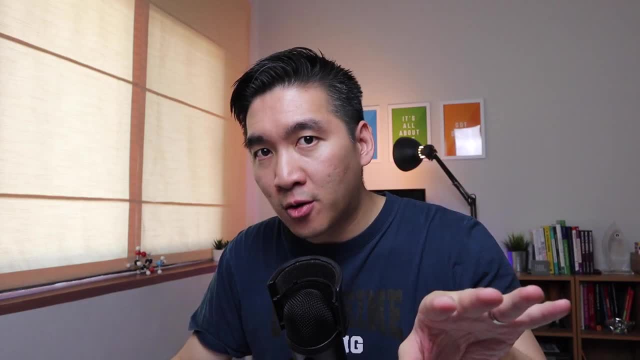 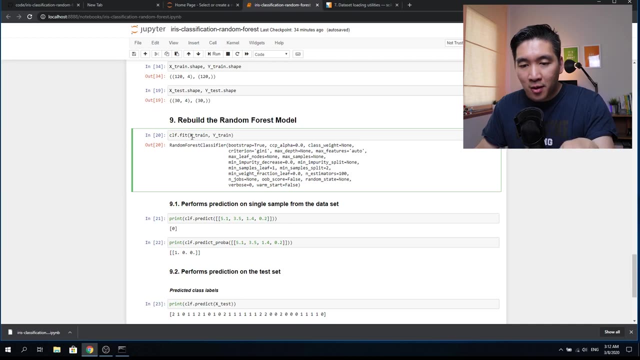 And so we're going to rebuild the classification model on this new train test split data. So we're going to use the CLF dot fit function where we define earlier that COF will refer to the random forest classifier, And then we're using default values for that And then the input argument to this function. 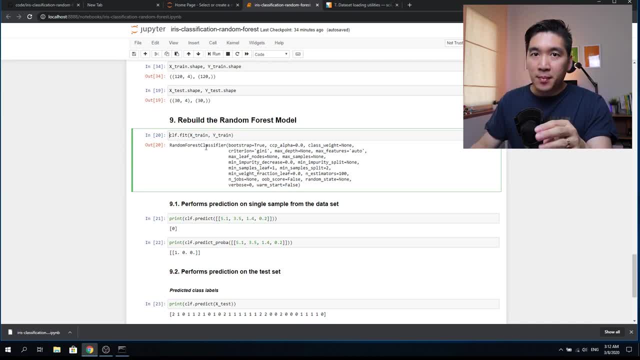 will be x train and y train. So it's going to specify the pairs of x and y for the training set, And then it's going to make a prediction afterward. So let's run the classification model, And so now the model is trained on the 80% of the data samples And then we're going to use 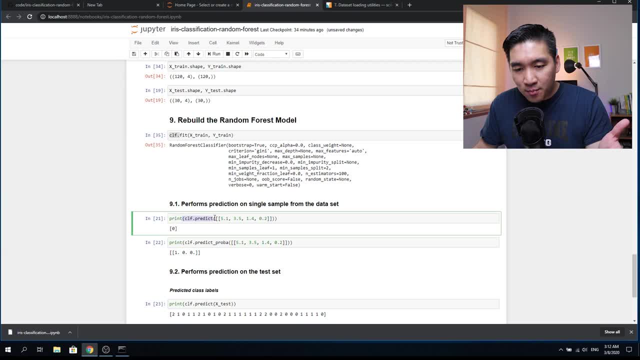 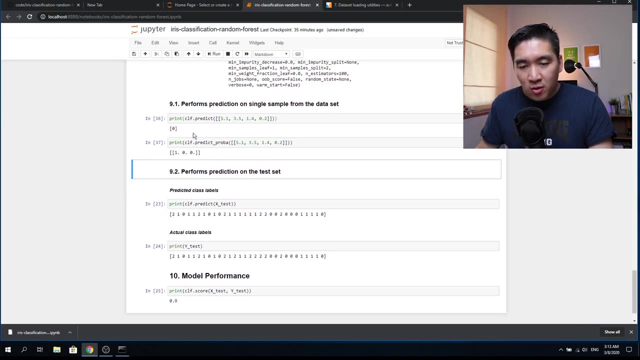 similar to the previous step. we're going to print the results of the prediction, where we're going to use the first flower as the input and then predict it out, and then the probability of the prediction. Okay, and so we get the same prediction that the first flower will be a iris citosa. 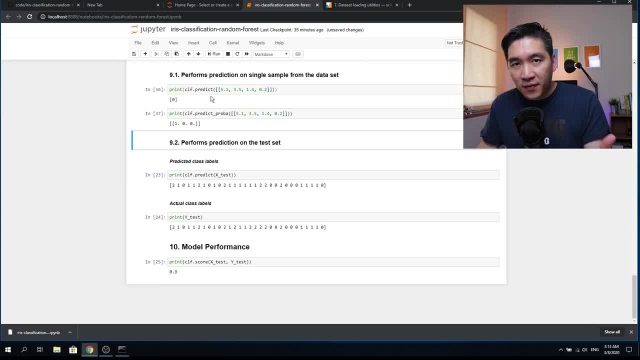 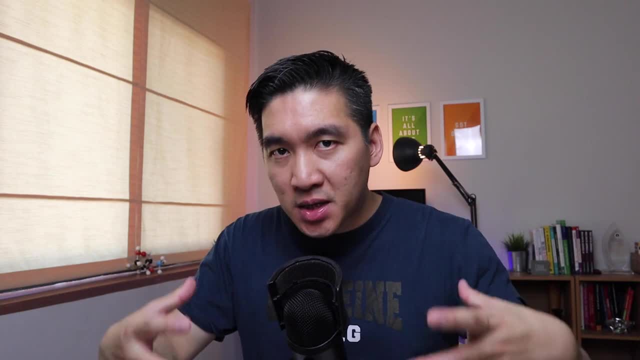 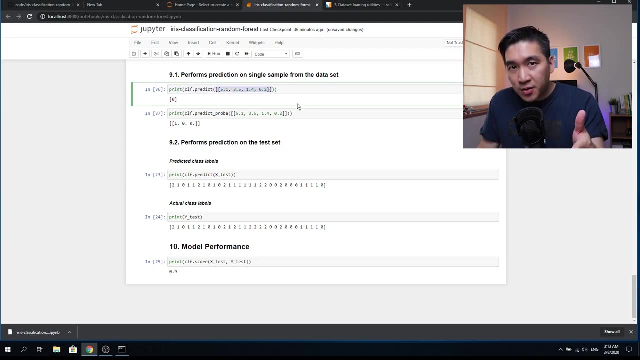 And so this is making a single prediction, meaning that we're feeding in the input values of one data sample. So let's say that we want to predict a set of samples containing more than one, So you can do that by, instead of using one set of features with four input values, we're going 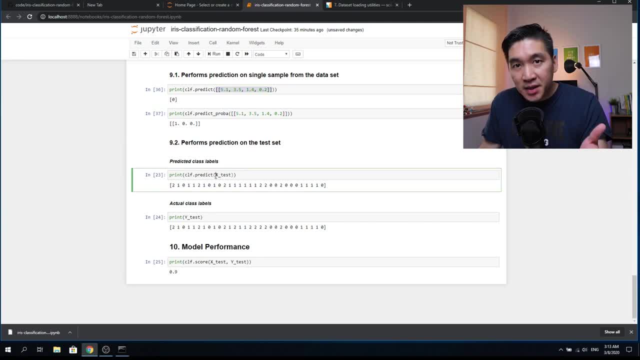 to use the whole data frame of the X test, which will comprise of 30 flowers. So, simply, we're going to use the print function And then we're going to print the results Of the CLF dot predict, and it's going to use the input argument of X test, And so that will give us. 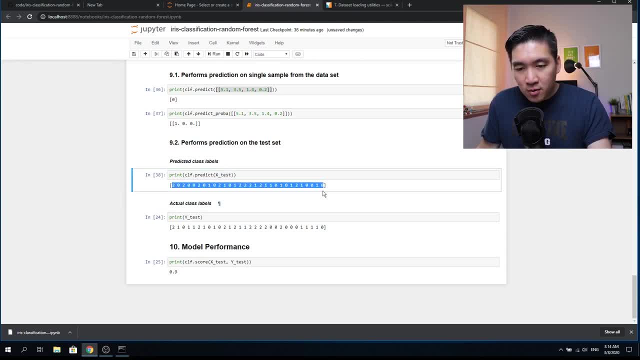 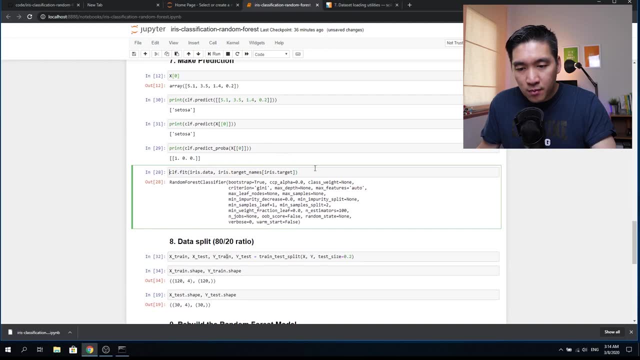 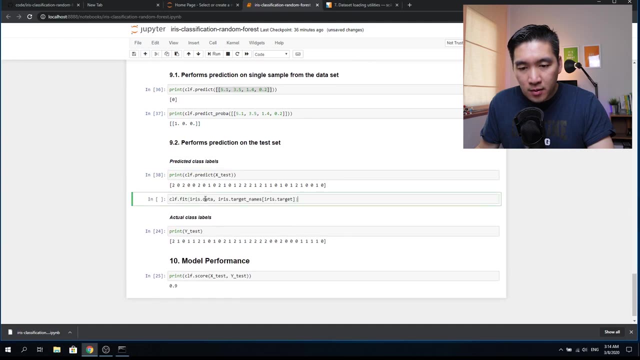 the prediction. So the predictions are shown here. And in order to see the test label, we're going to use the above lines of code here. We're going to copy that. Add a cell, put it below here, Okay, and then we're going to run it. 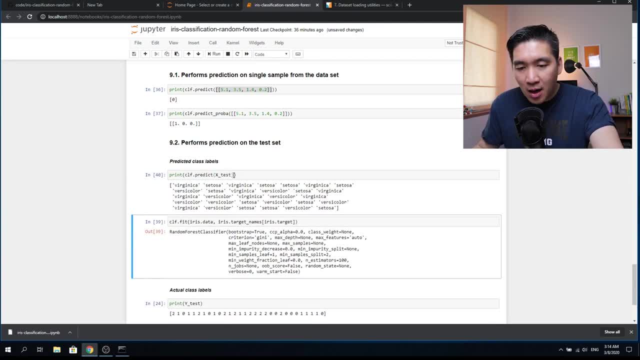 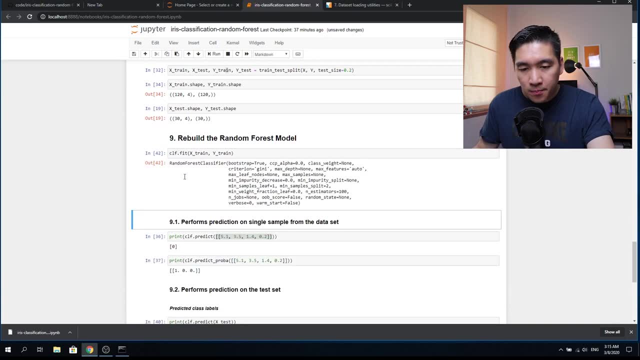 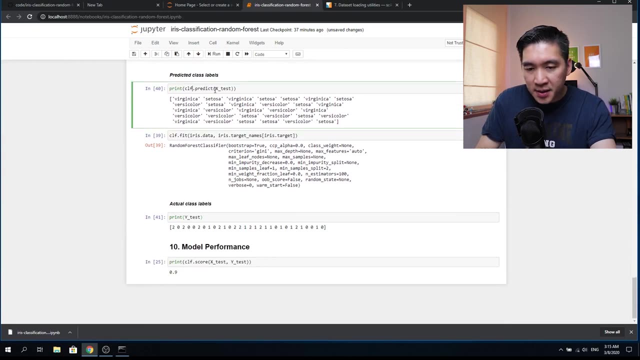 Okay, and then we're going to perform the prediction again, And now we're going to see the prediction as the class labels. So let's reboot the model again And perform the prediction on the X test again, And it will give us a series of values here, And so let's compare it with the actual. 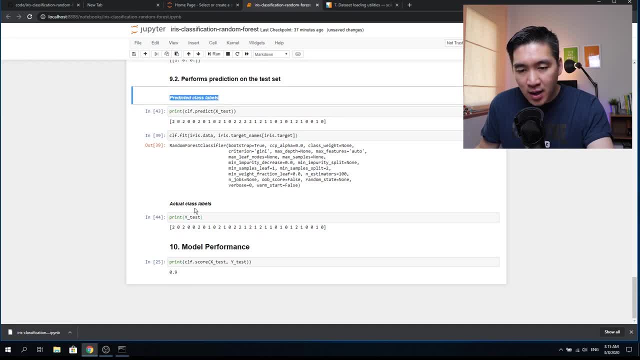 values. So this is the predicted values for the label And this is the actual class label. So we're going to see that in the first data sample it is predicted to be two, but it is also a two right in reality is zero here is predicted to be a zero if it's a two is 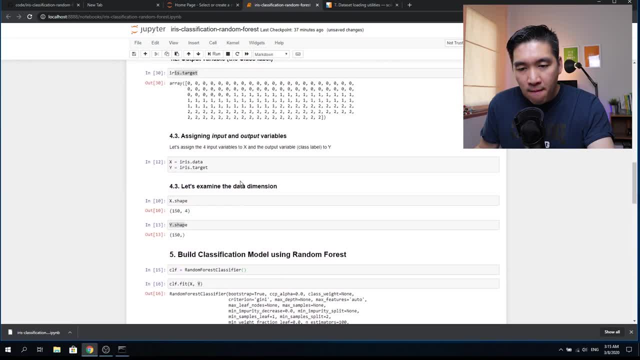 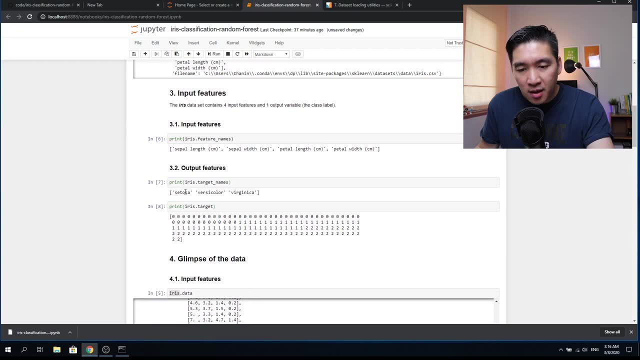 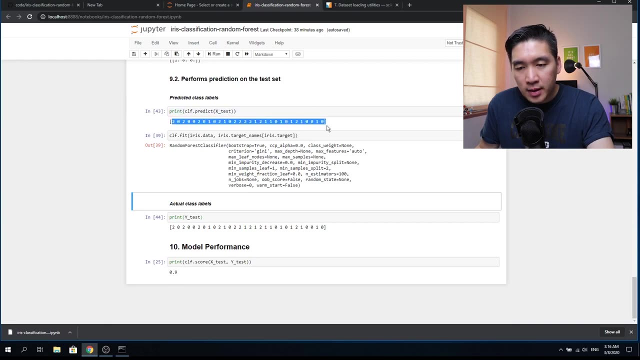 predicted to be a two. two meaning the values here Right Zero One. two corresponding to Setosa versus color and virginica. So you can see it in one goal. Okay, So you can see it in one goal D: the predicted values and the actual values. And then the last step in this Jupyter Notebook file. 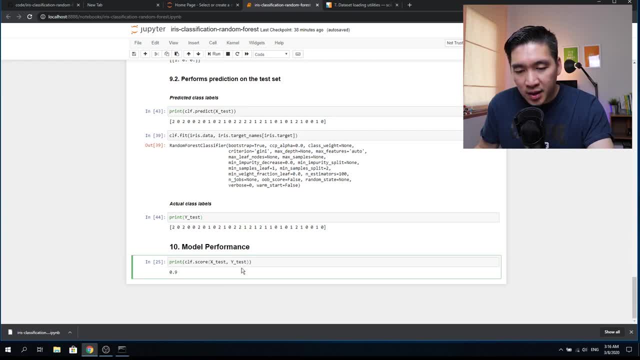 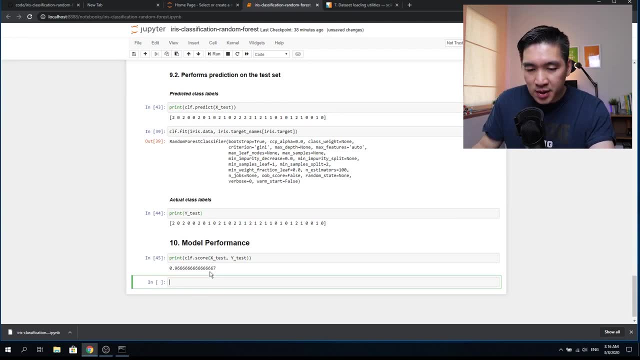 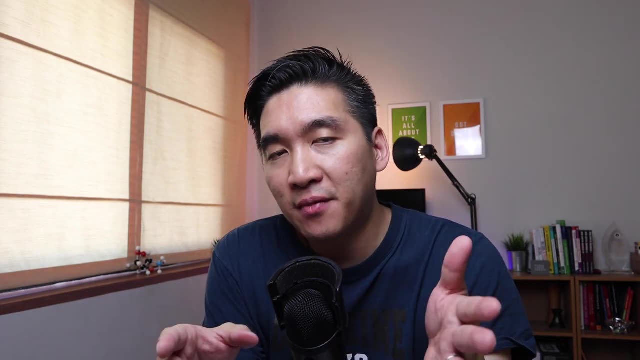 is to print the prediction score, which is the accuracy of the model, And it's take the input as the x test and y test And then it will output the score of 0.96.. So 96% accurate here. So congratulations. you have built your first classification model on the iris data set. 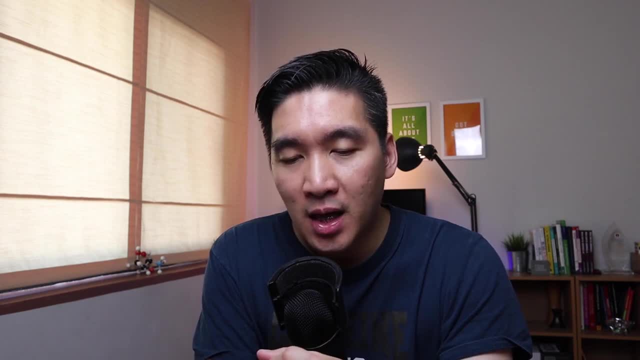 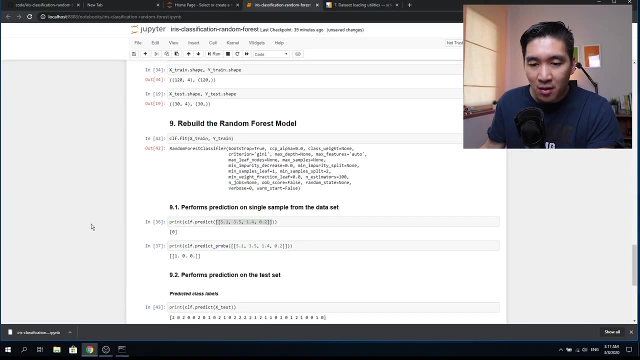 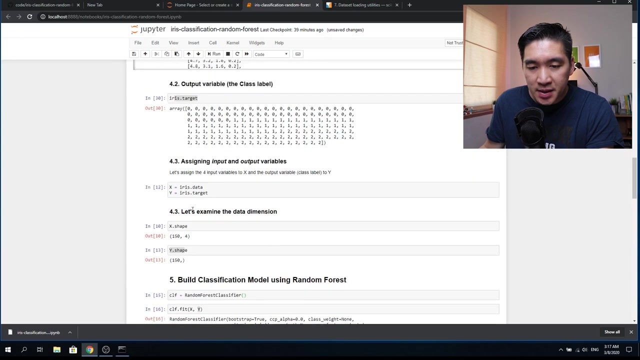 using the random forest algorithm, And so, in the meantime, before we release the next video, if you want to test out this with a new data set, please feel free to do so. So let me tell you how you can do that. Okay, so you're going to do it right here. instead of assigning x to be. 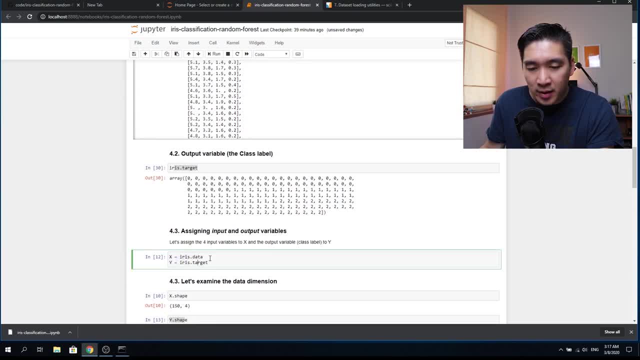 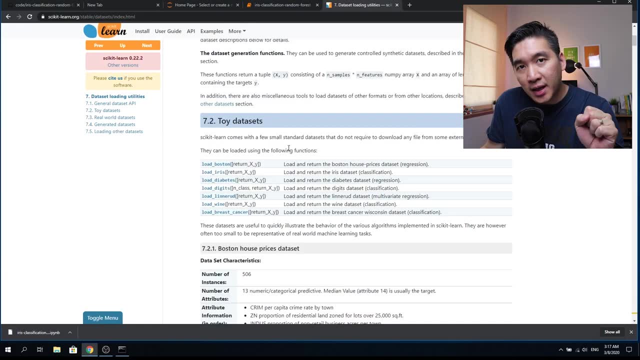 iris dot data and y to be iris dot target. you're going to use a different data set. Okay, And so let's see which data set are available for you to use. So scikit learn comes with a couple of toy data set. So the first one that we use was the iris data set, And so the other data sets are. 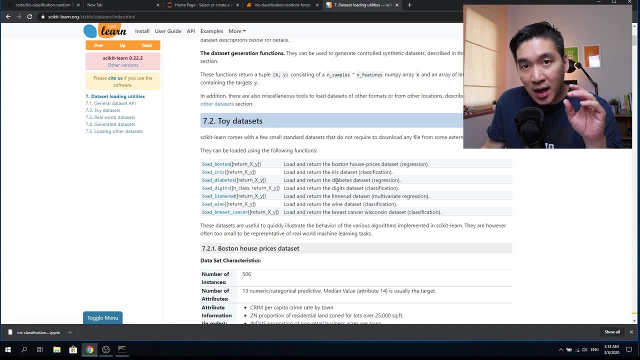 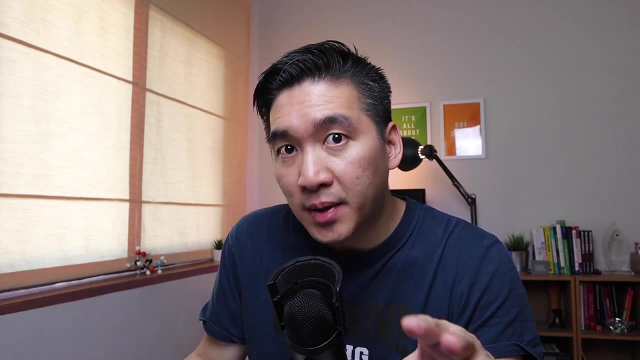 shown here. they have the Boston house price data set, the diabetes data set and several others, So please check it out And in the next tutorial we're probably going to use some of these as an examples And if you would like to suggest some data set as examples to use in future videos. 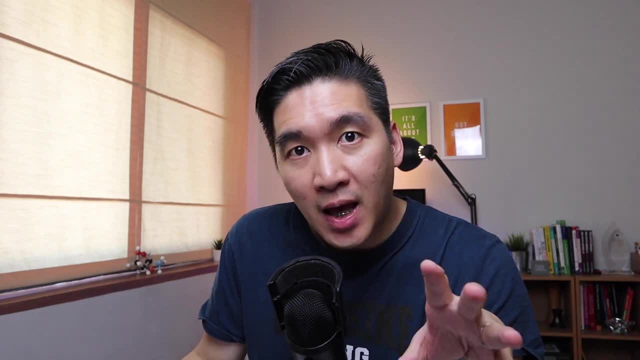 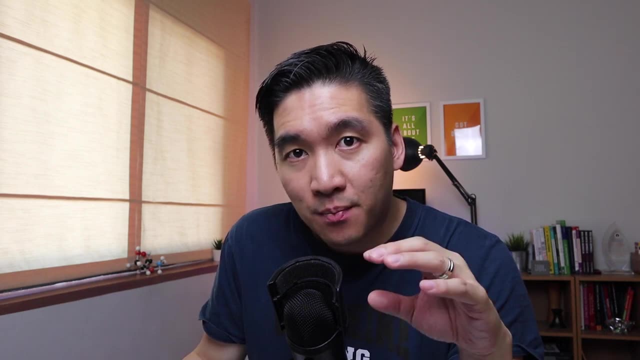 please do so by commenting down below, And please don't forget to to try it out with a different data set and save your project And we'll see you in the next video. Bye for now. progress by uploading it to your GitHub profile And, as before, the best way to learn data science. 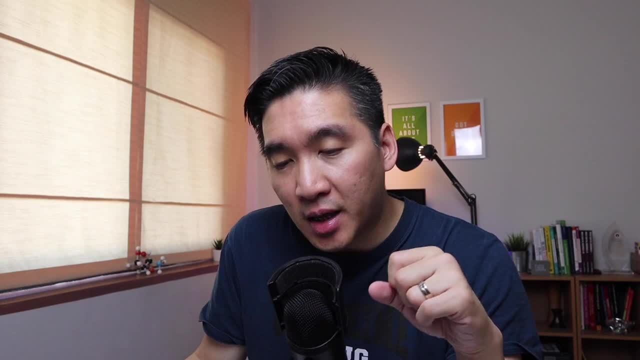 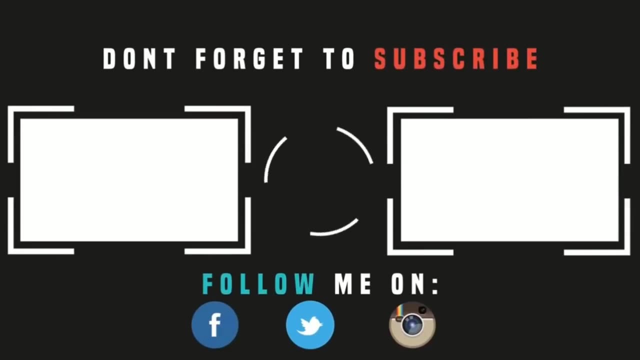 is to do data science. So until next time, I'll see you in the next video. Thank you for watching. Please like, subscribe and share, And I'll see you in the next one, But in the meantime, please check out these videos.